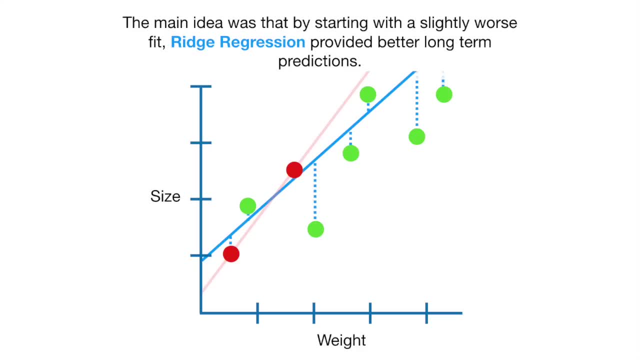 The main idea was that, by starting with a slightly worse fit, ridge regression provided better long-term predictions. Bam, Now let's go back to the equation that ridge regression minimizes and focus on the ridge regression penalty. If, instead of squaring the slope, we take the absolute value, then we have lasso regression. 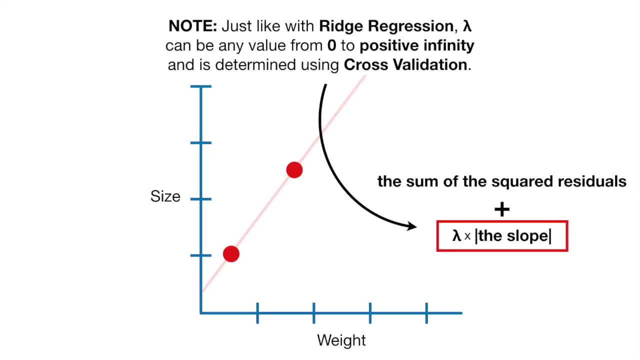 Note: Just like with ridge regression, lambda can be any value from 0 to positive infinity and is determined using cross-validation. Like ridge regression, lasso regression, the orange line results in a line with a little bit of bias, But less variance than least squares. 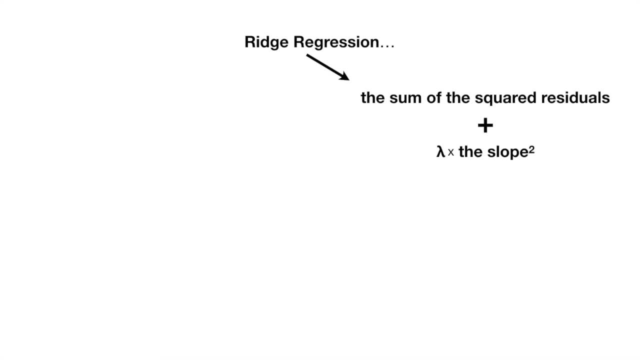 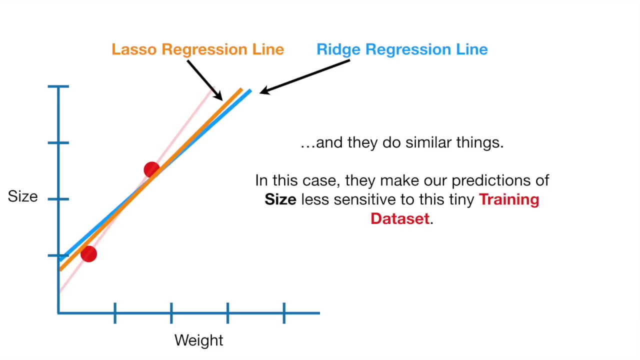 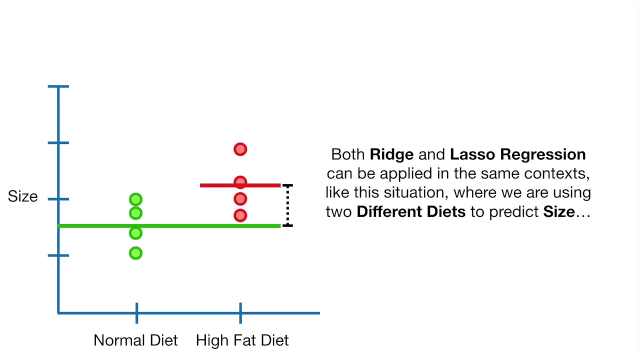 Bam Ridge regression and lasso regression look very similar And they do similar things. In this case, they make our predictions of size less sensitive to this tiny training data set. Both ridge and lasso regression can be applied in the same context, like this situation where we are using two different diets to predict size. 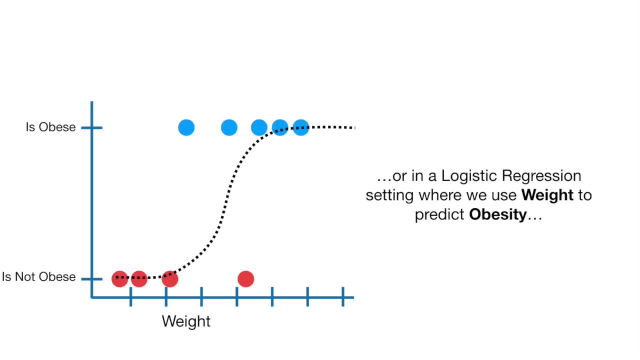 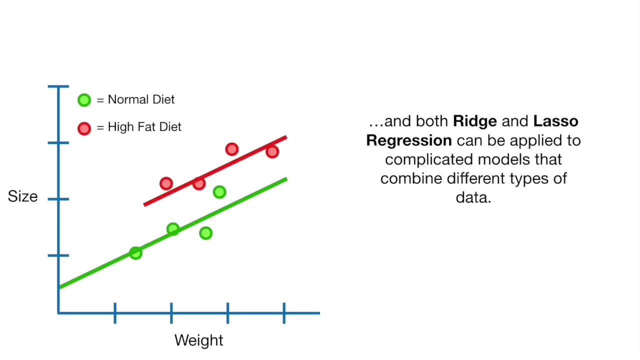 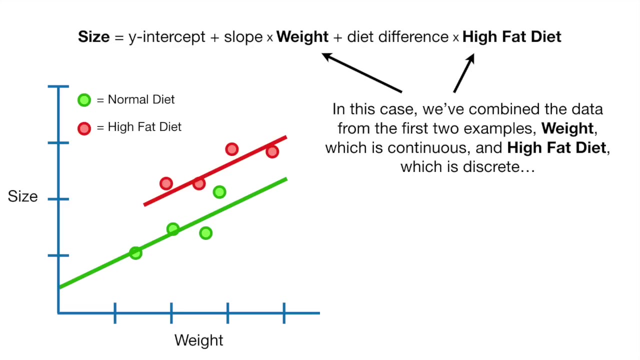 Or in a logistic regression setting where we use weight to predict obesity, And both ridge and lasso regression can be applied to complicated measurements. In this case, we've combined the data from the first two examples: weight, which is continuous, and high-fat diet, which is discrete. 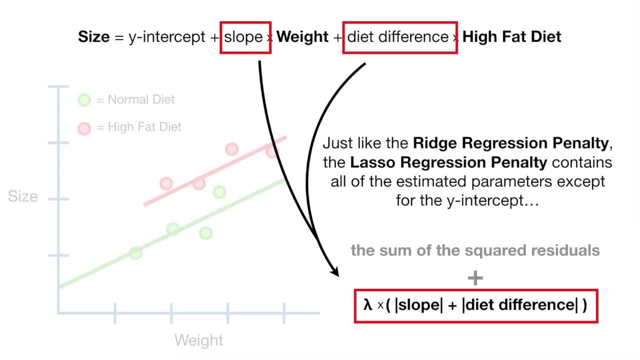 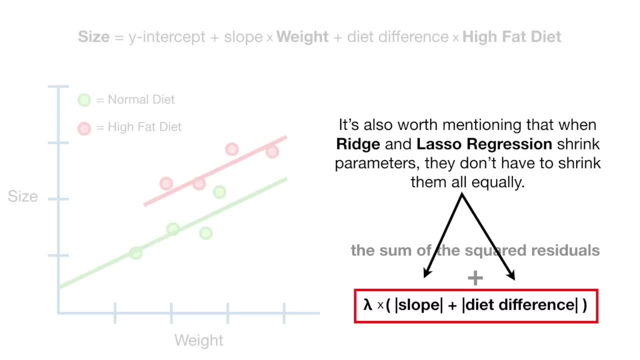 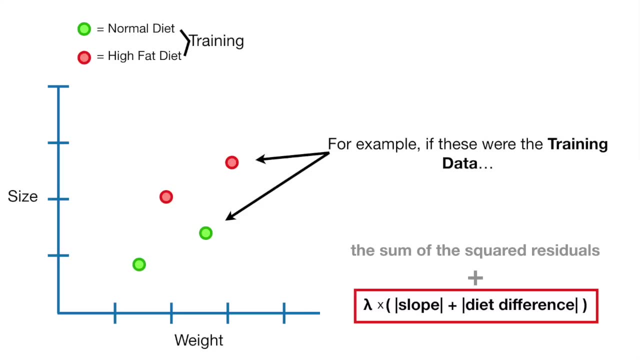 Just like the ridge regression penalty, the lasso regression penalty contains all of the estimated parameters except for the y-intercept. It's also worth mentioning that when ridge and lasso regression shrink parameters, they don't have to shrink them all equally, For example, if these were the training data. 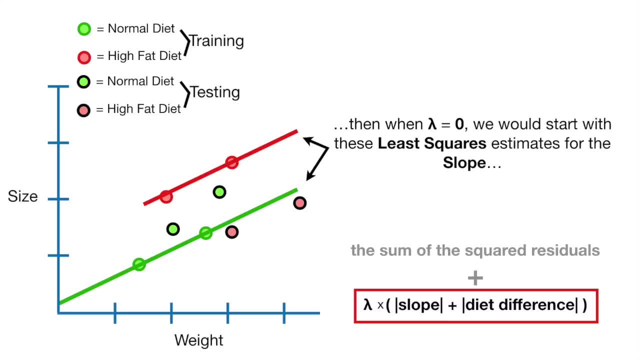 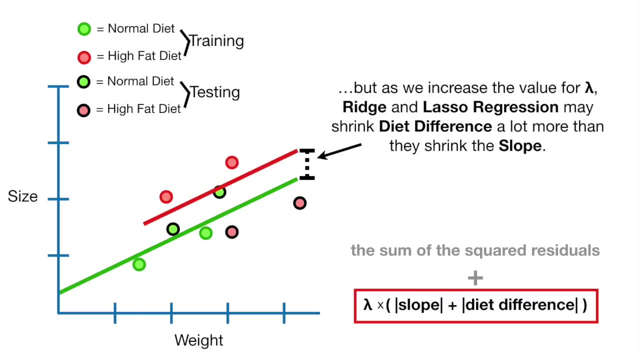 and these were the testing data. then, when lambda equals zero, we would start with these least squares estimates for the slope and the offset for diet difference. But as we increase the value for lambda, ridge and lasso regression may shrink diet difference a lot more than they shrink the slope. 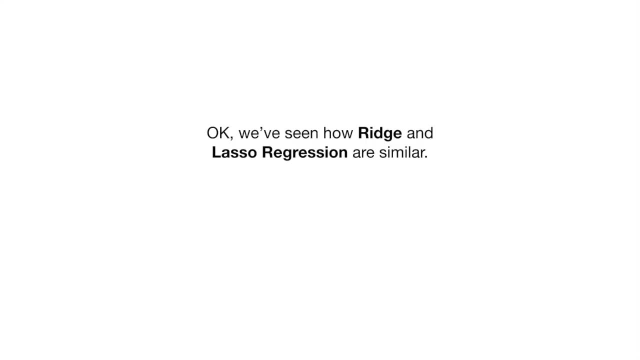 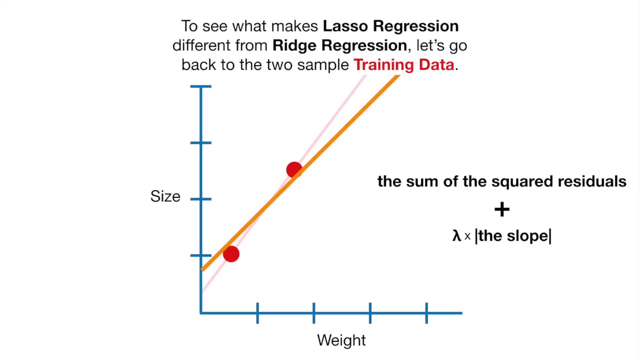 Okay, we've seen how ridge and lasso regression are similar. Now let's talk about the big difference between them. To see what makes lasso regression different from ridge regression, let's go back to the two sample training data And let's focus on what happens when we increase the value for lambda. 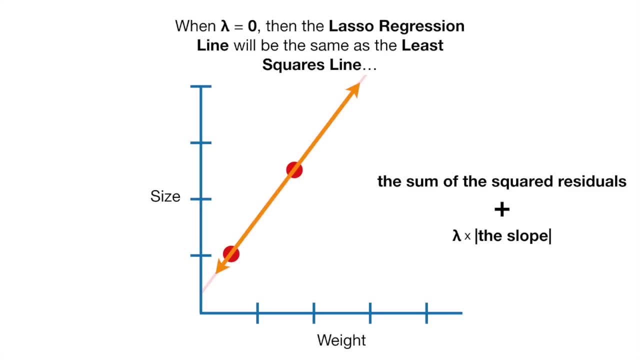 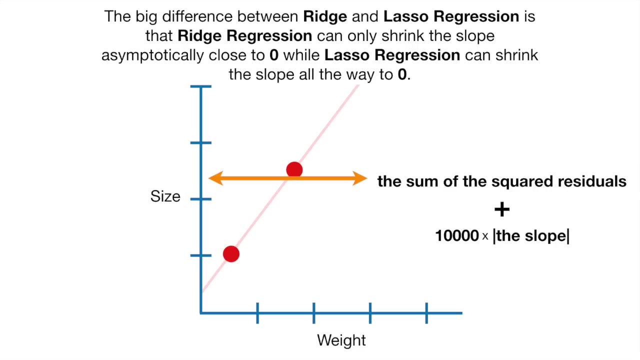 When lambda equals zero, then the lasso regression line will be the same as the least square. As lambda increases in value, the slope gets smaller, Until the slope equals zero Bam. The big difference between ridge and lasso regression is that ridge regression can only shrink the slope asymptotically close to zero. 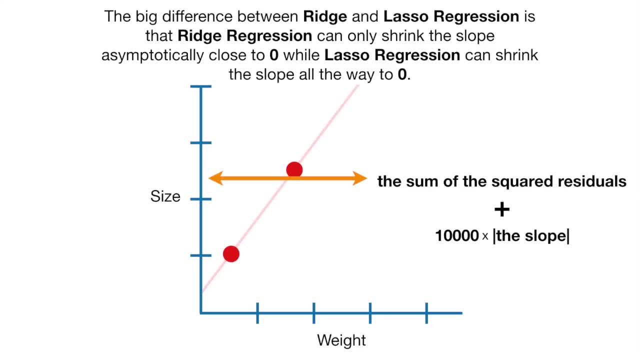 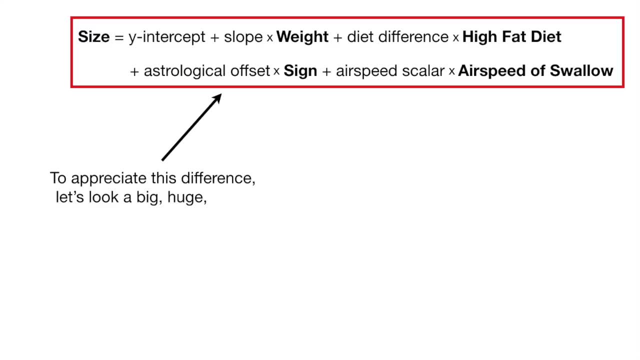 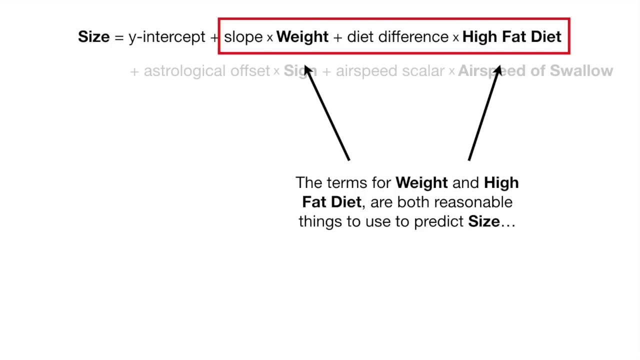 while lasso regression can shrink the slope all the way to zero. To appreciate this difference, let's look at a big, huge, crazy equation. The goal of this equation is to predict size. The terms for weight and high fat diet are both reasonable things to use to predict size. 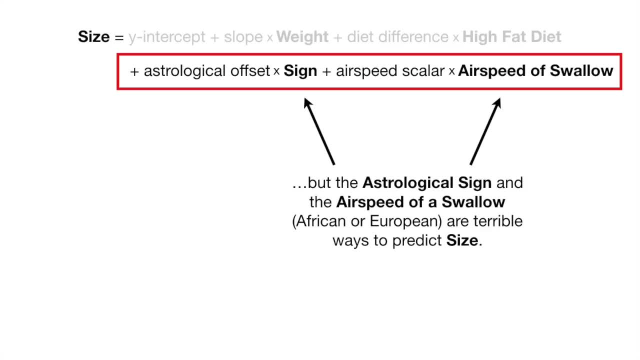 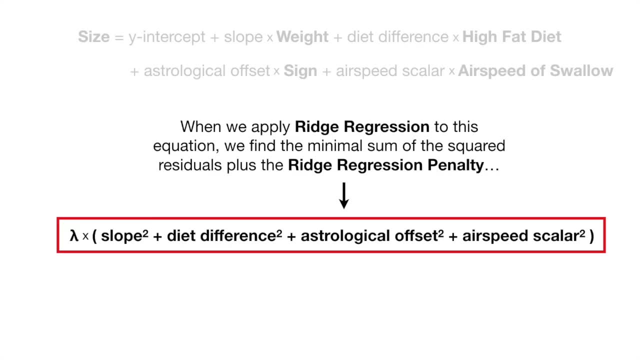 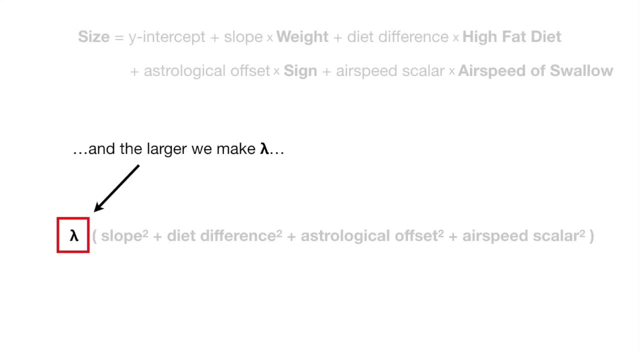 But the astrological sign and the airspeed of a swallow are terrible ways to predict size. When we apply ridge regression to this equation, we find the minimal sum of the squared residuals plus the ridge regression penalty, And the larger we make lambda, these parameters might shrink a little bit. 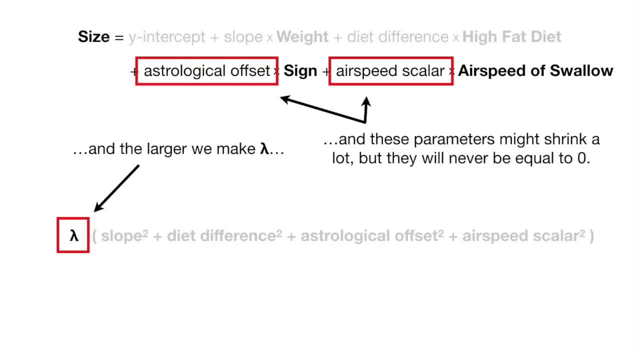 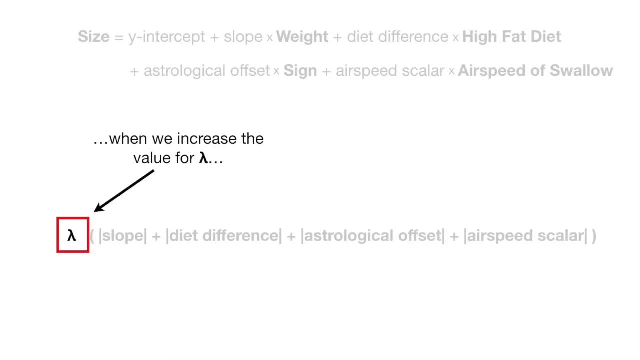 and these parameters might shrink a lot, but they will never be equal to zero, In contrast with lasso regression. when we increase the value for lambda, then these parameters will shrink a little bit and these parameters will go all the way to zero. 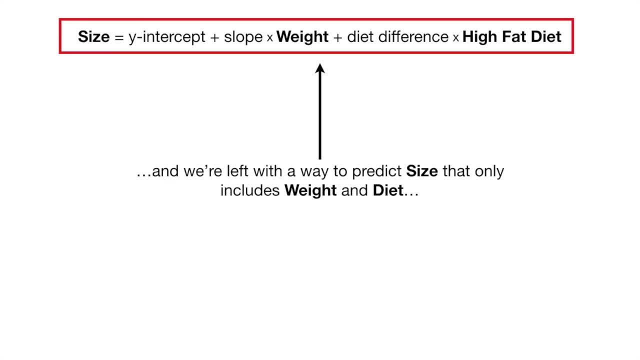 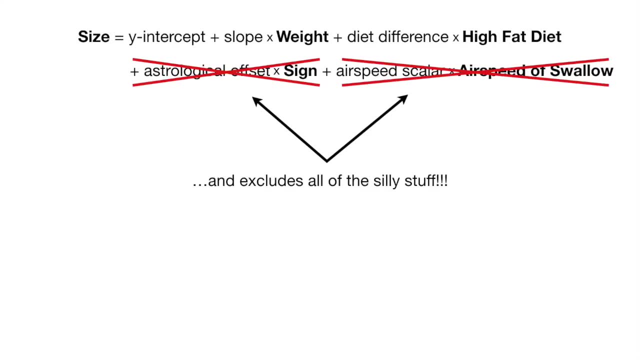 and these terms go away and we're left with a way to predict size that only includes weight and diet and excludes all of the silly stuff. Since lasso regression can exclude useless variables from equations, it is a little better than ridge regression at reducing the variance in models that contain a lot of useless variables.